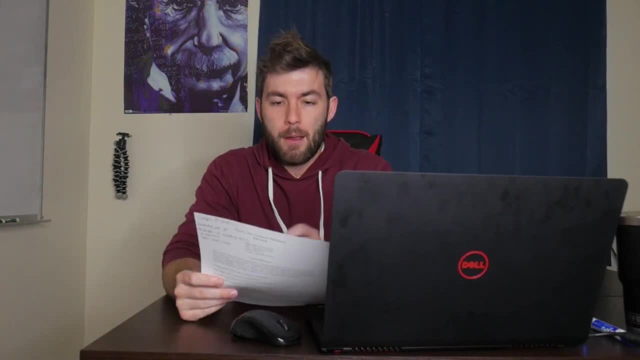 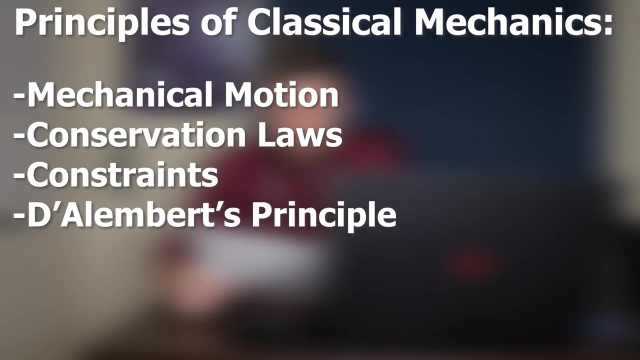 which we didn't get to, But let's go ahead and get started. Number one: principles of classical mechanics, which entailed mechanical motion conservation laws, constraints, and de Lambert's principle. This was- uh, this is basically just pre-Lagrange. 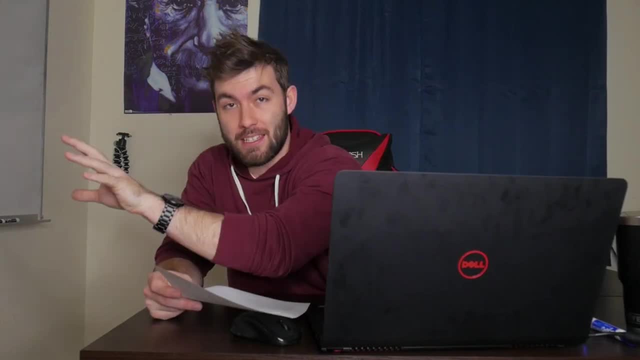 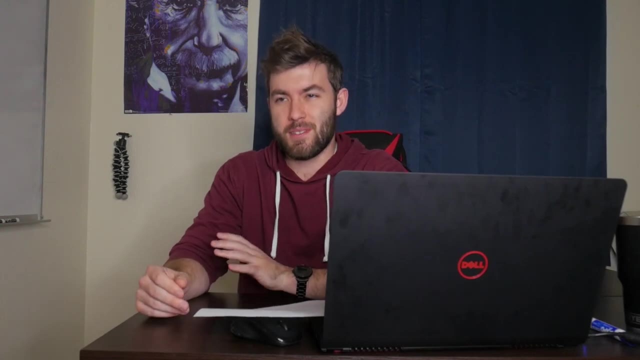 And Hamiltonian stuff just almost getting to that. um, especially with the de Lambert's principle, That was something that I initially struggled with quite a bit, because it introduces concepts like virtual work and virtual displacement, which didn't really make sense to me at the time. 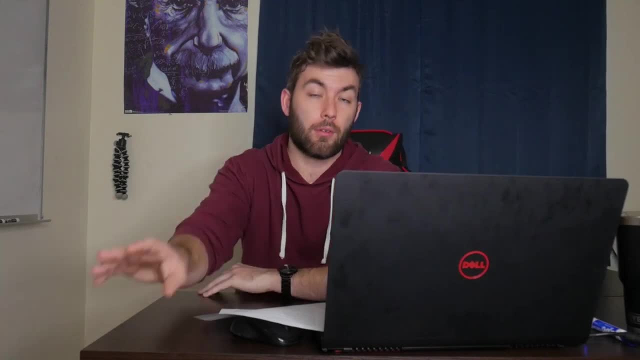 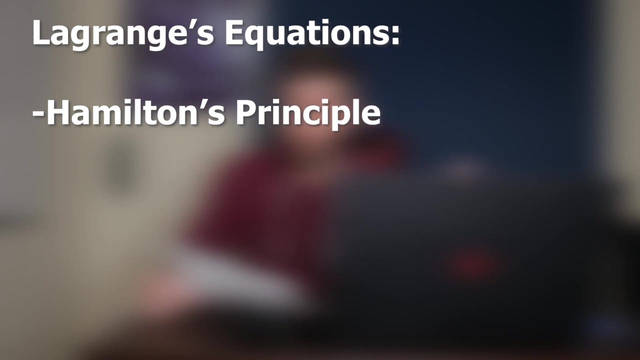 But you can use de Lambert's principle to derive the Lagrangian formalism, and that's actually what we get into next, uh, which is Lagrange's equation. So with that we had Hamilton's principle, variational methods, Lagrange's equations of motion. 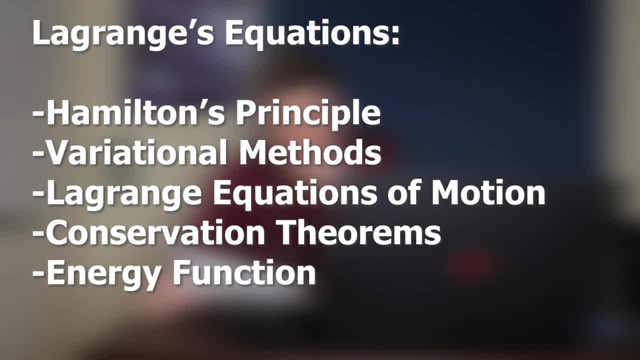 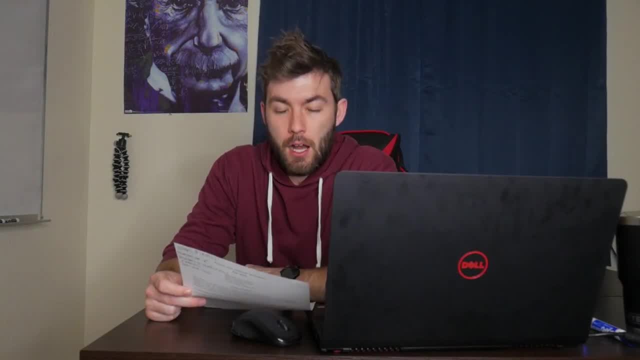 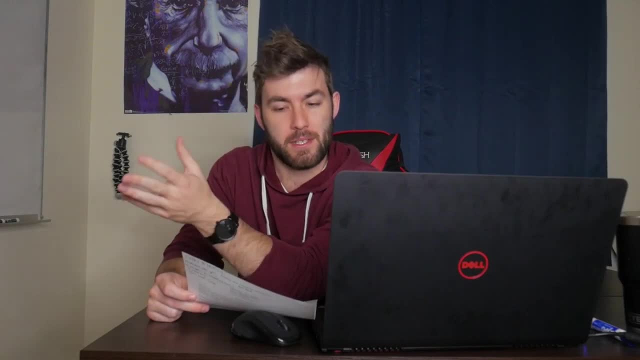 conservation theorems and the energy function, Hamilton's principle. basically, you can use the principle of least action, which tells you how lazy nature is, uh, to use that as a secondary way of deriving Lagrange's equations of motion or the, the Lagrangian formalism as a whole. 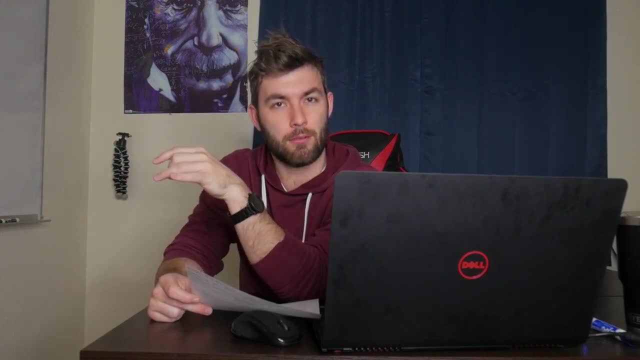 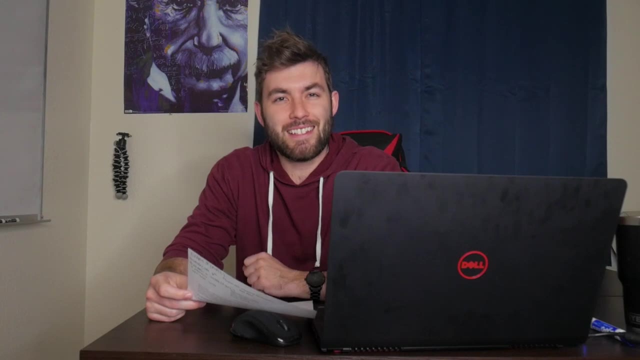 That one made much more sense to me. It was easier, I think, to derive the Lagrange equations using Hamilton's principle versus de Lambert's principle. But you know, to each their own, I guess, Variational methods, that's kind of just the method you use. 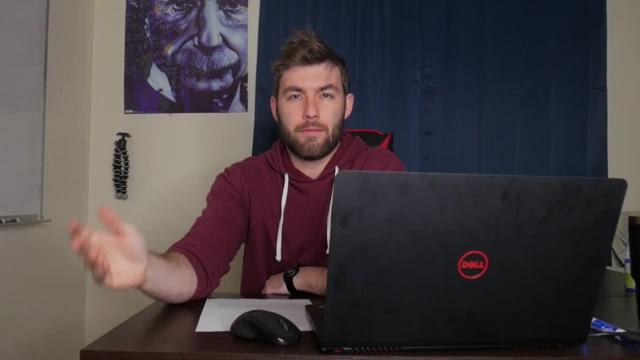 To get to that, Lagrange's equations of motion. I've made videos on. If you're really interested in it, I'll leave links in the description so that you can see maybe some examples of that. But they're. they're systems of partial differential equations in terms of what are. 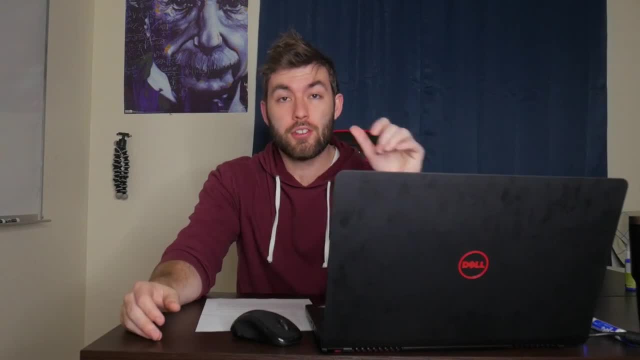 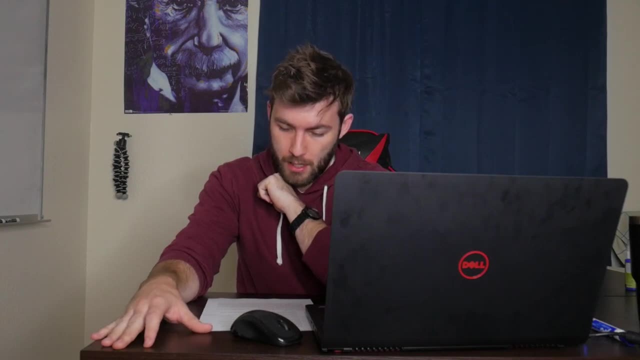 called generalized coordinates and velocities. They're the Lagrangian version of f, equals ma They give you your equations of motion. Um, then we got into- just lost my place- uh, conservation theorems and the energy function. Now, when I was an undergrad, we didn't get into, uh, Lagrangian. 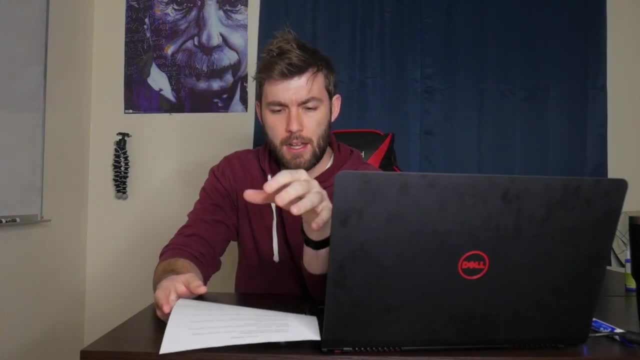 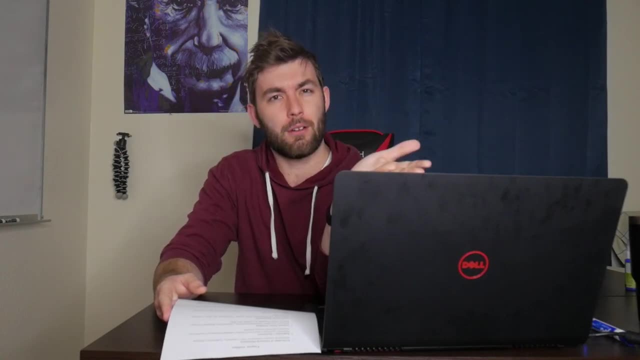 until towards the very end of the semester, Whereas for this class we basically kicked things off with it. There was probably a week or so that we did- uh, you know, effectively a review, like center of mass coordinates, that kind of stuff, But then we went straight into Lagrangians. 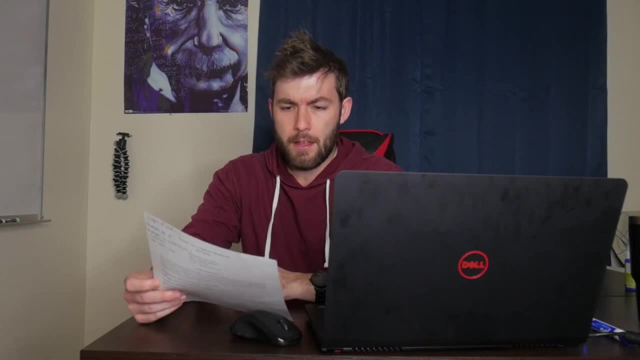 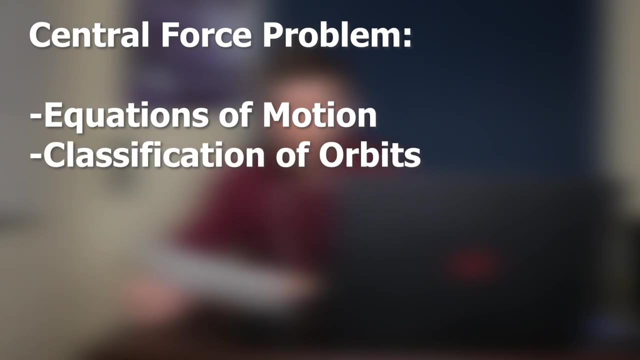 and we stayed with Lagrangians for a while. Um, the next one was the central force problem, which encompassed equations of motion, That's pretty vague- Classification of orbits, virial theorem, Bertrand's theorem, Kepler's laws scattering in a central. 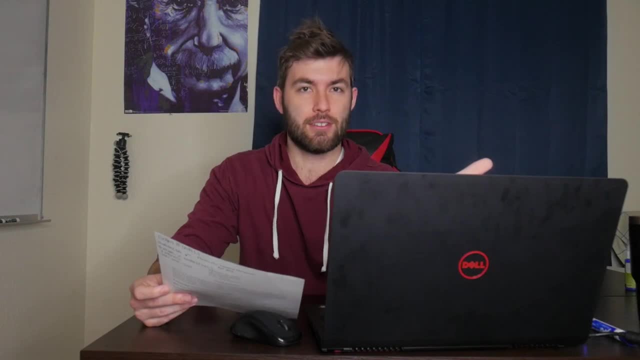 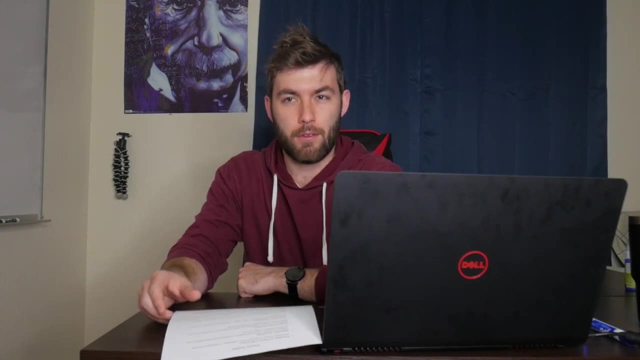 force field. So you can probably tell by context here that this had a lot to do with, uh, orbital mechanics. This was probably the hardest section for me, to be honest. It just seemed like a lot to keep track of for the different types of orbits, whether you got parabolic, elliptic, 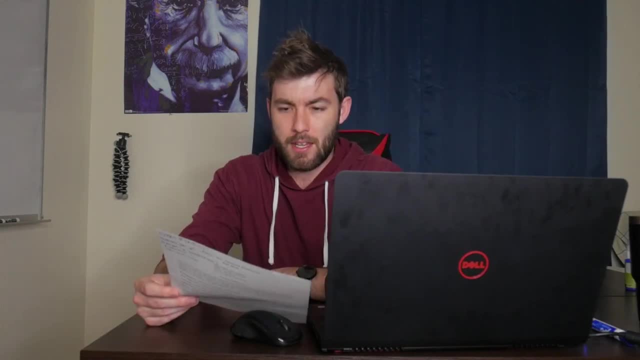 hyperbolic circular orbits. So, uh, I wasn't too fond of this section. If there was one that I would go back to in my free time, it'll probably be this one, just because, uh, you know, it's probably a. 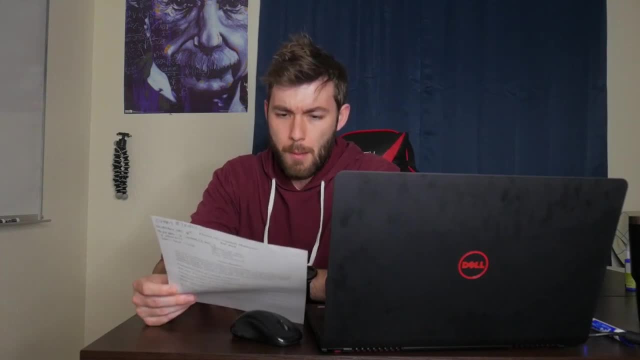 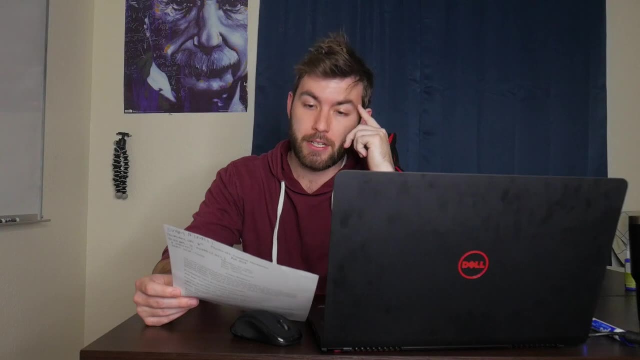 weak point of mine that I need to like work on a little bit. But we also went into, uh, scattering force fields, so we went over things like differential cross sections. I liked that section a lot. That actually had a lot to do with my senior thesis. Uh, so it's it's. I should be. 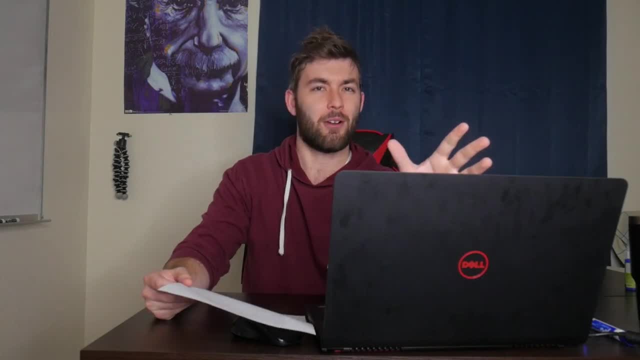 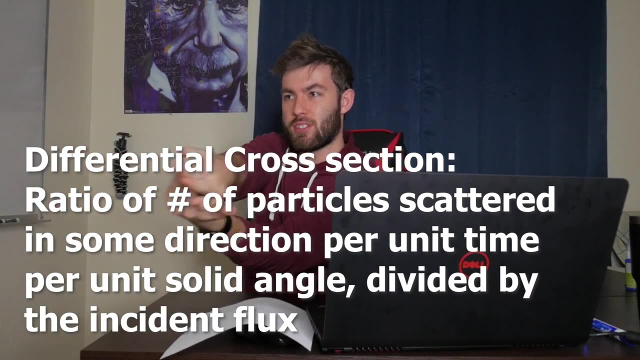 careful, but it's basically measuring probability in units of area. sometimes It's like: uh, if you have scattering, what's the probability of getting an amount of particles in this angle swept? Definitely an interesting section. Then we get into rigid body kinematics. uh, orthogonal. 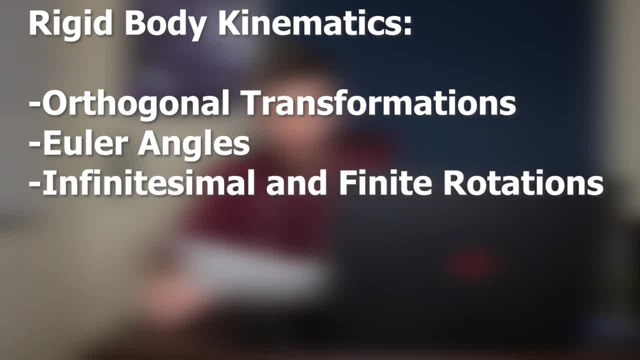 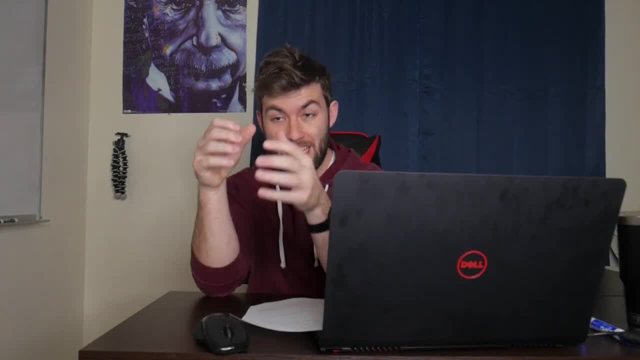 transformations, Euler angles, infinitesimal and finite rotations and the Coriolis effect. Euler angles were pretty cool, Like, say, you have a reference frame of the system or in the system that you're interested in, so if you're watching someone fly through the air and then you go to 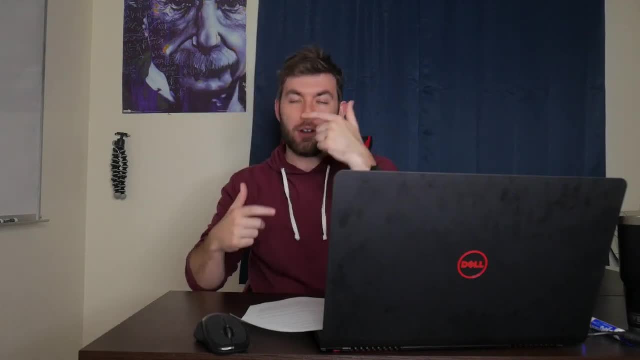 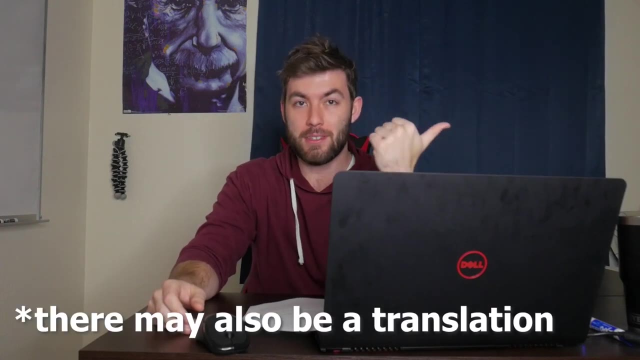 their reference frame of them going through the air. the way of converting in between those are through Euler angles, so it's a bunch of rotating your axes to get into the same frame. So you have your body frame and the lab frame and then in between you have an intermediate frame, so there's 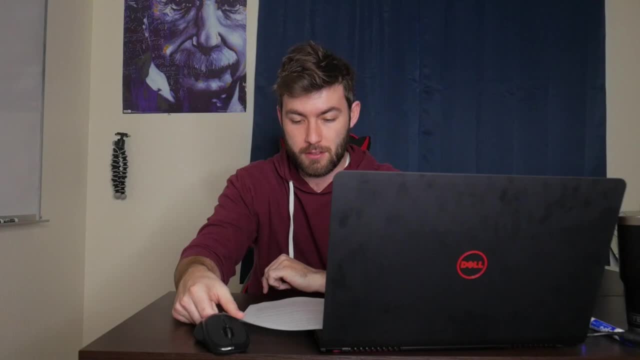 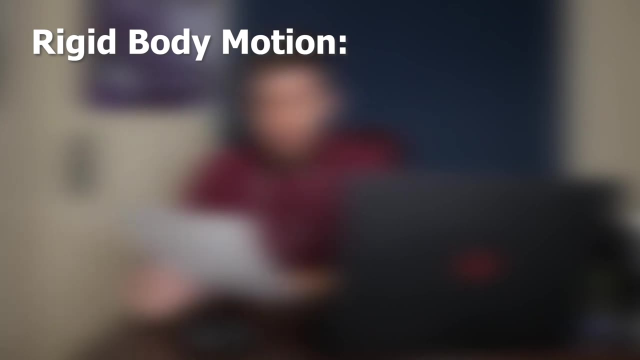 typically three rotations, I should say generally three rotations associated with it. I thought that was the fun part. and then, yeah, the Coriolis effect. Moving on to rigid body motion, Sounds a lot like rigid body kinematics, I know, but we went over angular momentum, the inertia tensor principal. 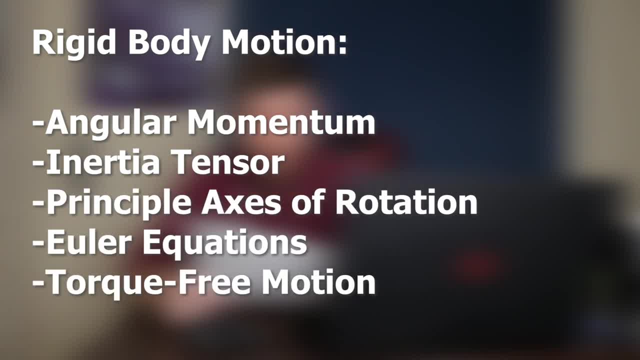 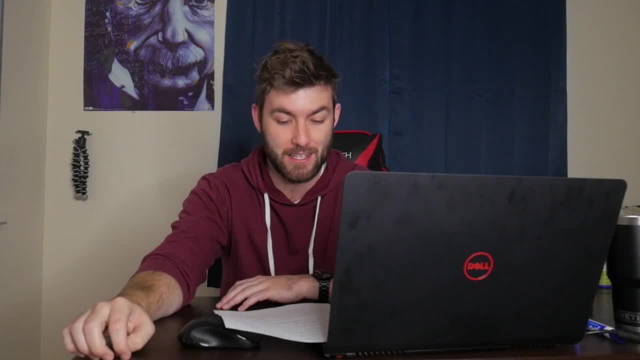 axes of rotation, Euler equations, torque-free motion and precession. I've pretty much beat the inertia tensor to a pulp these past few weeks on my channel, so I'm not going to be getting that into that again here. I'll leave a link in the description if you're curious about it. Um. 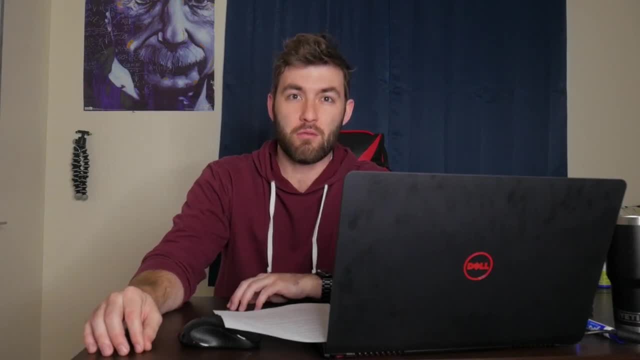 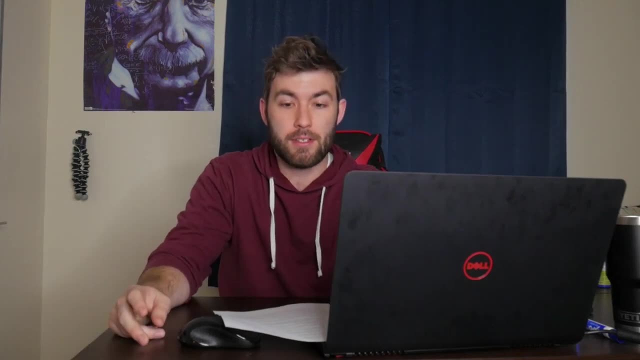 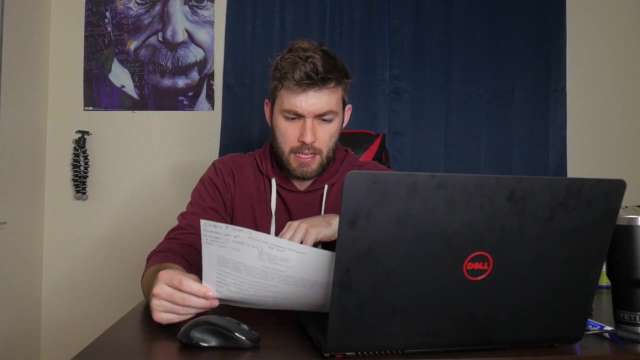 principal axes of rotation. basically, in this chapter we got really good at describing how things spin. We went over like the, the symmetric spinning top gyroscopes, all that good stuff. It basically means: uh, I am the most dangerous person on Earth with a Beyblade. Next is Hamilton's equation. so 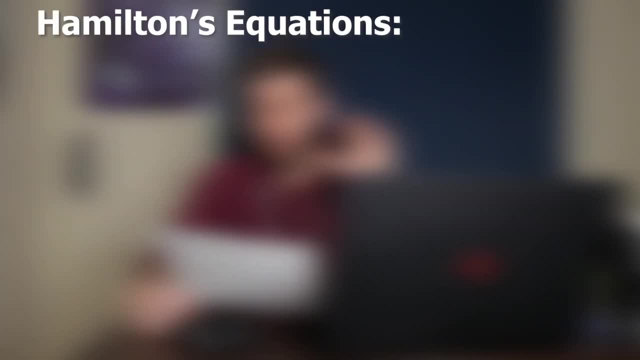 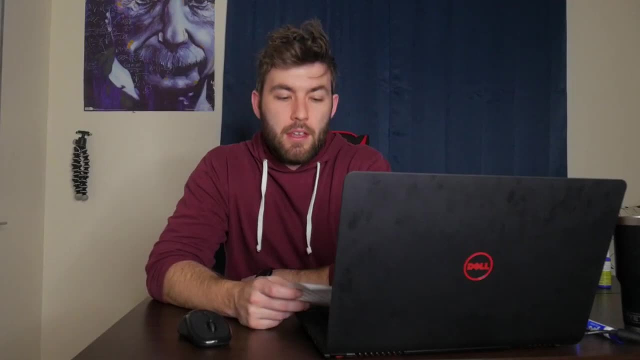 the next chapter. we're finally getting into the Hamiltonian formalism. We went over Legendre, transforms uh, Hamilton's equations of motion, conservation theorems and the principle of least action. The Hamiltonian formalism you might be familiar with if you've had any quantum mechanics. 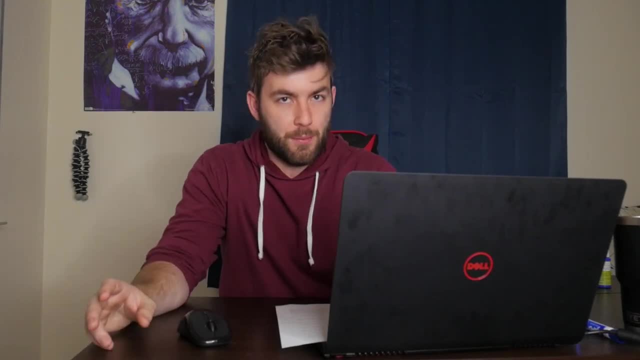 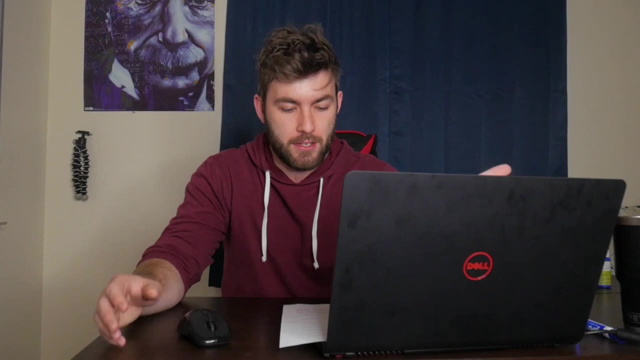 and it's connected to the Lagrangian through a laser Legendre transformation. You'll be familiar with Legendre transformations if you've had any thermo and statistical mechanics, if you've seen like TDS equations. Basically it takes, it connects. 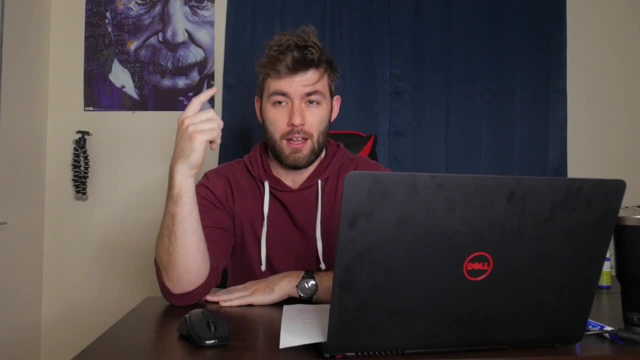 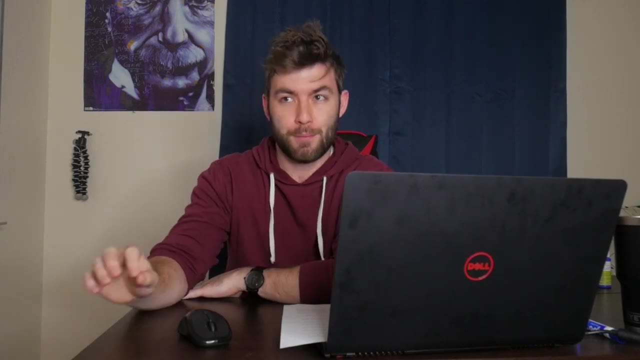 a, uh, a variable with its conjugate. So for example, uh, generalized velocity and the generalized momentum. The generalized momentum in general is not as simple as just multiplying by the mass, multiplying the generalized velocity by the mass. You've got to be more careful than that, Um so 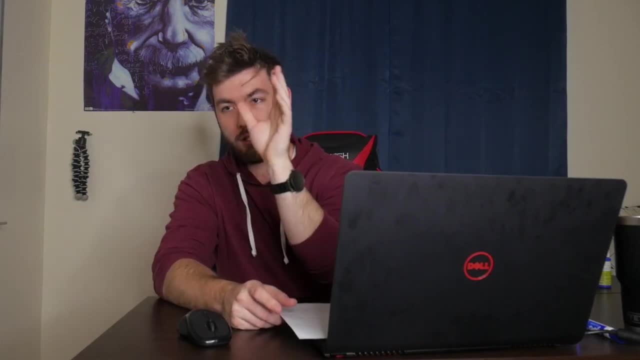 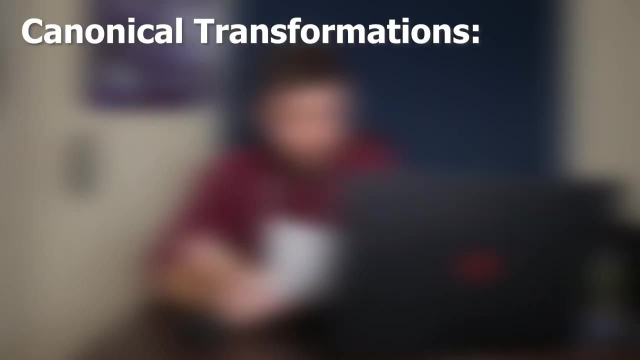 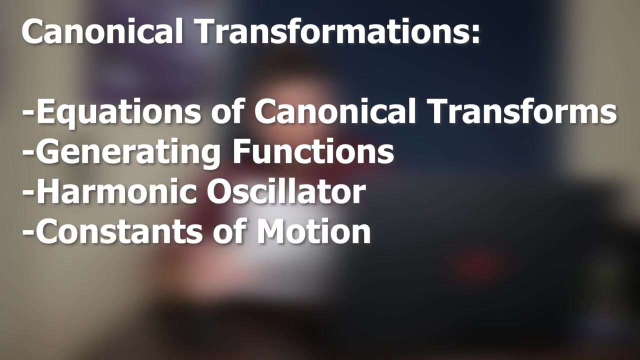 they're connected to the Legendre: transform, We create or we construct the whole Hamiltonian formalism, and I already talked about the principle of least action. Moving on to canonical transformations, Equations of canonical transformations, Generating functions, harmonic oscillator constants of motion, Poisson brackets, Louisville theorem, Hamilton-Jacobi equation: 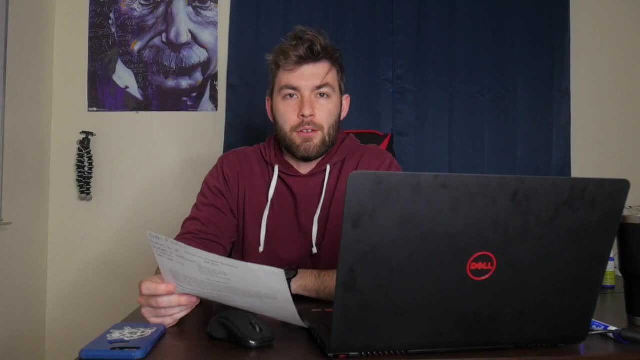 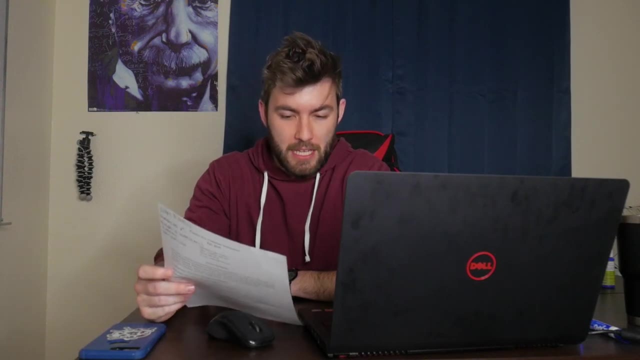 and Hamilton's characteristic function. This section was actually pretty new territory for me. We really didn't go over this in undergrad and frankly I think it would be kind of a lot to do in undergraduate. classical mechanics, Uh, so I'm not really at a point. 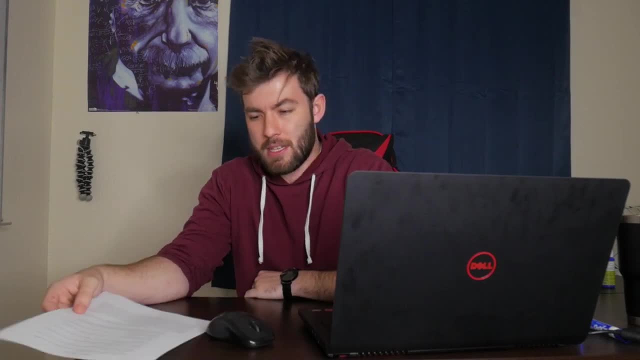 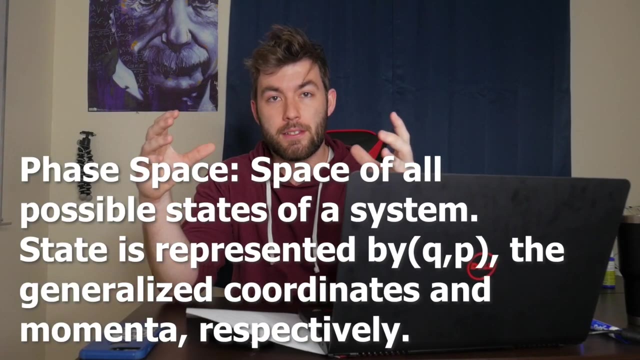 where I can explain this stuff simply. so I'm sorry, But to even begin going over canonical transformations you have to be comfortable with the concept of phase space, And points in phase space are a collection of the generalized coordinates and generalized momenta, And in this 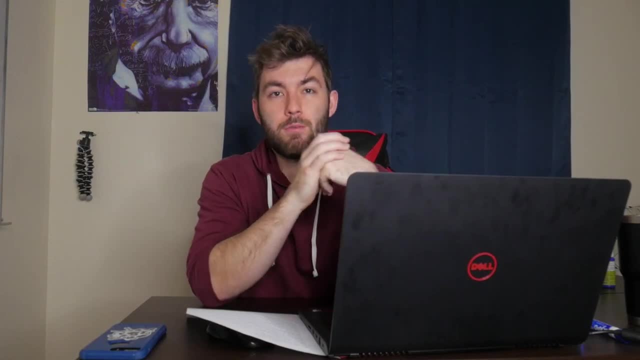 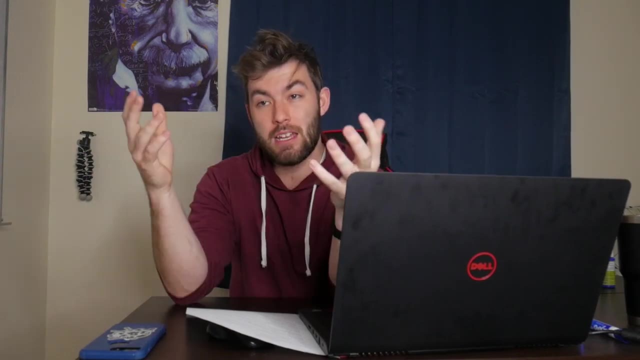 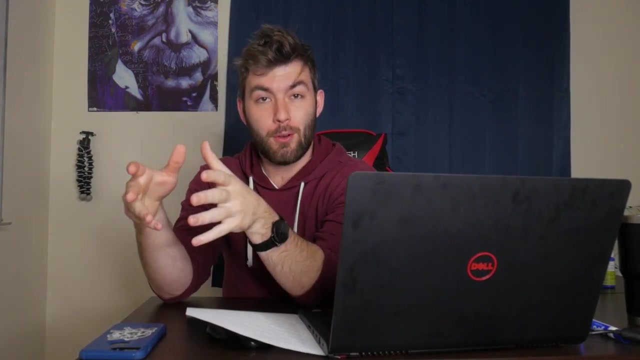 phase space, you can do transformations, And transformations which preserve sort of the form of the Hamiltonian are called canonical transformations. And if you want to say transform the coordinate and the momenta, then you'll get these terms that are in terms of the old Hamiltonian, the new Hamiltonian, which is sometimes denoted k.